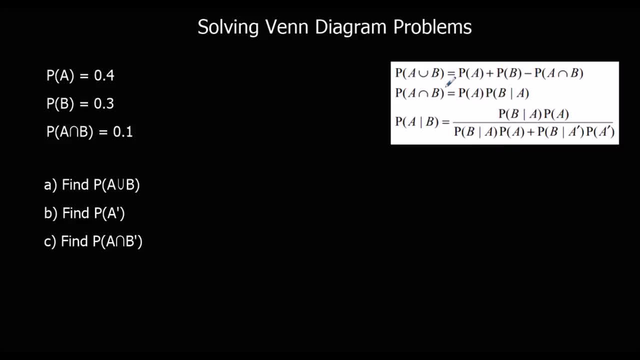 given to us in the formula book, which I've put a copy of here. I don't really use them very much. I use the first one. So the probability of the union of A and B is the probability of A plus the probability of B minus the probability of A and B, And we 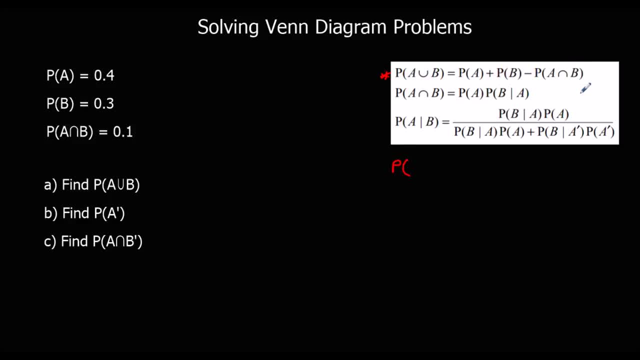 can also rearrange it by adding the probability of A and B to both sides and subtracting the probability of the union of A and B, which has the effect of switching them over. There you go. Amazing değil, Tom. So that means the probability of A and B is the 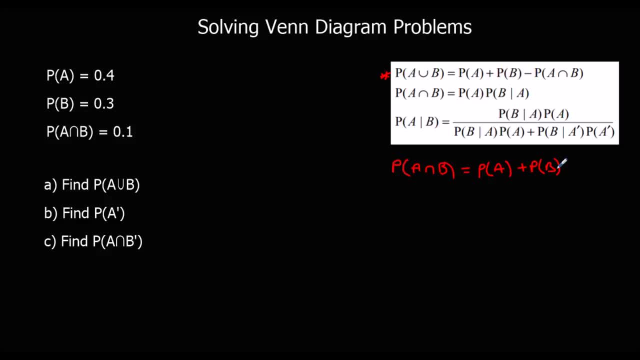 probability of A plus the probability of B minus the probability of B minus the probability of the union of A and B, The given that formula. So this B line means the probability of B given A. It certainly makes the difference between the two ender lines of the здесь. 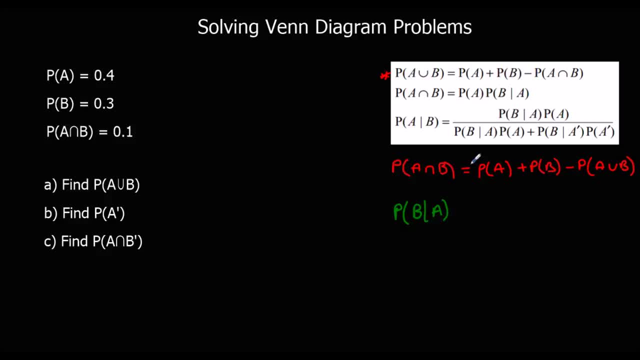 ArgiEs, If we have the probability of B given A, Here we have a line that says A- This is a rearranged version of this one. it's the probability of both of them together. so a and b, or b and a, divided by whatever's given. so for a given that question, you divide by whatever's given. 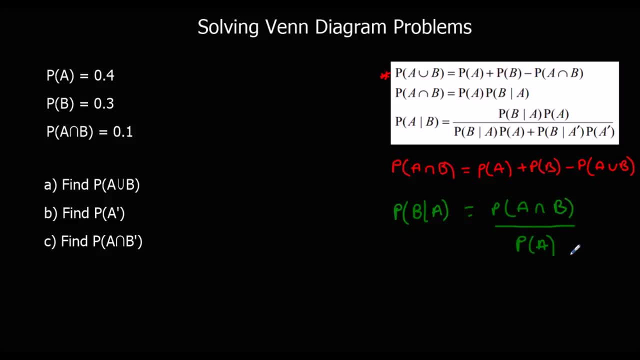 so a is given, so it's divided by the probability of a. if it was the probability of a given b and b is given, it'll be the probability of both of them together divided by the probability of b. so these are the formulas that we're actually going to be using. 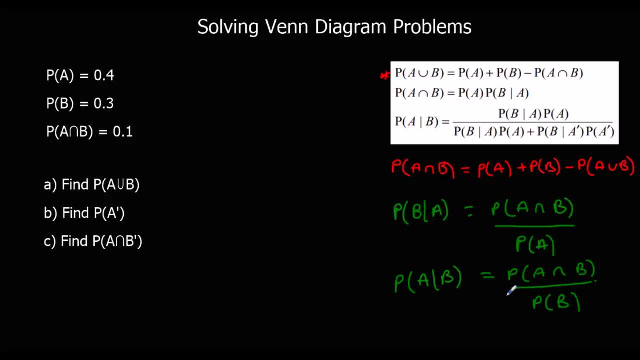 answering these questions. so here we've got some information and this information is enough for us to draw our venn diagram. so we've got a and b for the two circles. these two circles are a and b- an a circle and a b circle. so a and b, that goes in the middle. 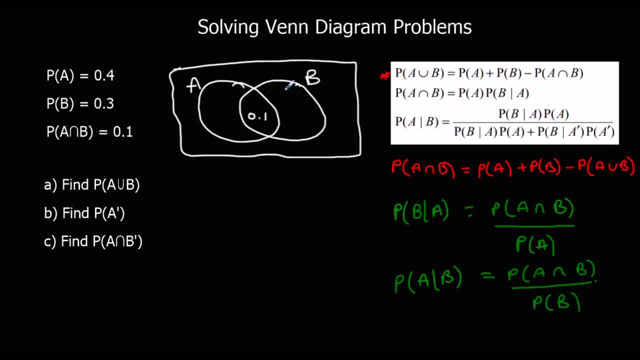 so the middle is the area that represents both a and b at the same time. the probability of a is 0.4. we've already got 0.1, so that means the rest of the circle must be 0.3. the probability of b is 0.3. 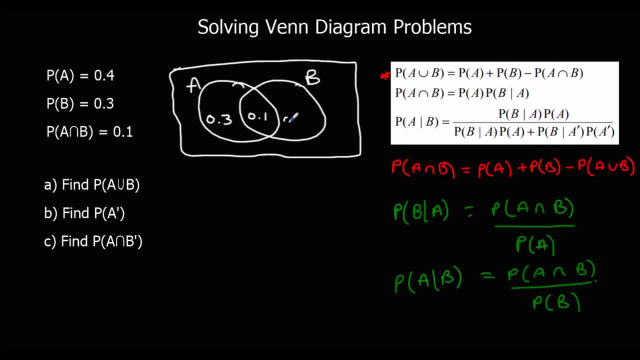 we've already got 0.1, 0.1 in the B circle, so we need another 0.2.. So far we've got 0.6, so outside. so neither A or B must be whatever's left to make it 1, because all probabilities add up to one. 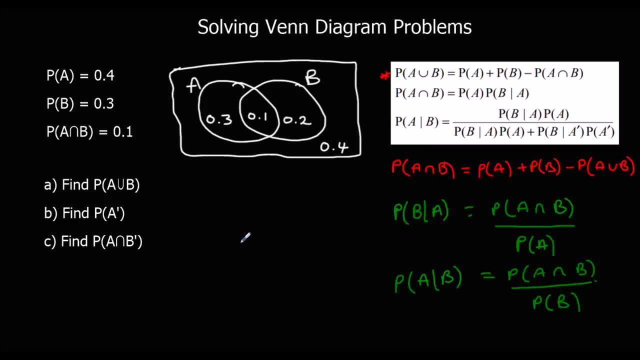 whole, the outside must be 0.4.. So the first question: find the probability of the union of A and B. So we could use this formula: the union of A and B, so 0.4 plus 0.3 minus. 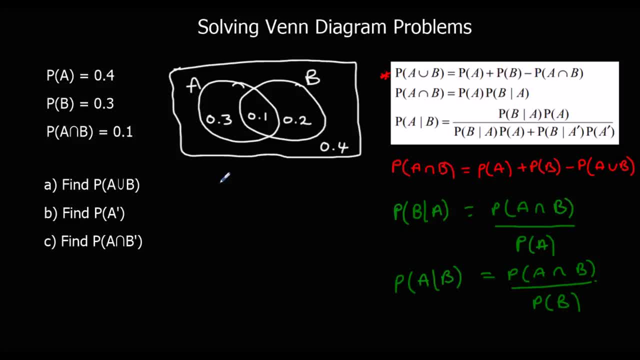 0.1,, which would be 0.6, or we could just look at our Venn diagram and say these two are A, these two are B, and a union means all of that. so all of those together and that's 0.6.. The probability of not A, that's everything that's not A. so we could do 1. 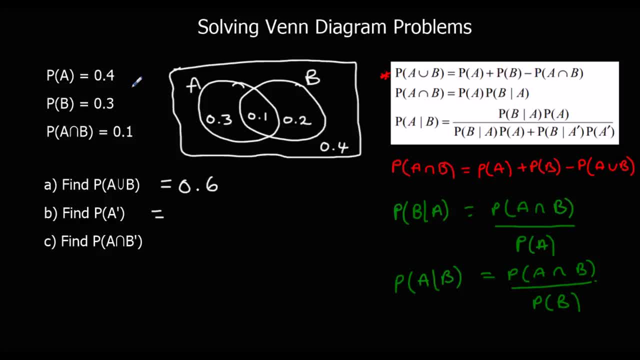 minus the probability of A, which is 0.6,. or we could just look at the ones on the Venn diagram that aren't A, which is 0.2, plus 0.4,, which is also 0.6.. And the probability of. 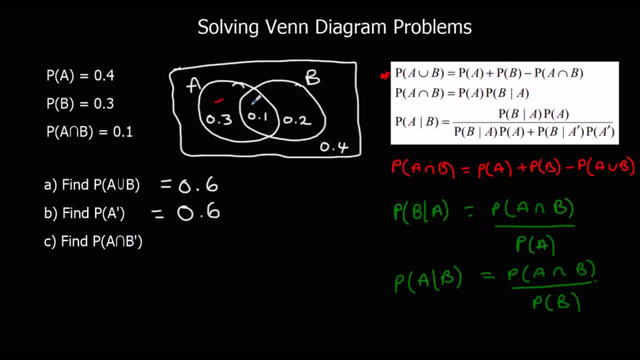 A is 0.6.. And not B. So these ones are A, which ones are not B? that's these two. So which ones are both of those? Where is it A and not B? It's the one with both the lines, so that's. 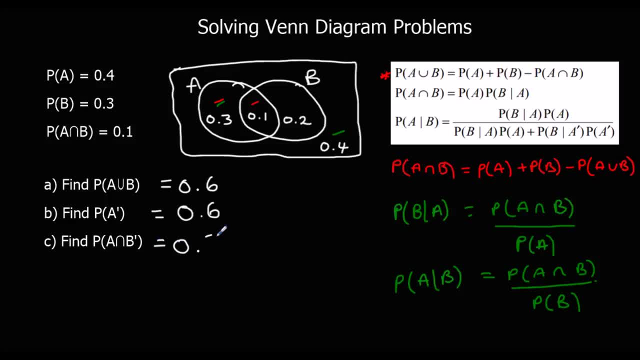 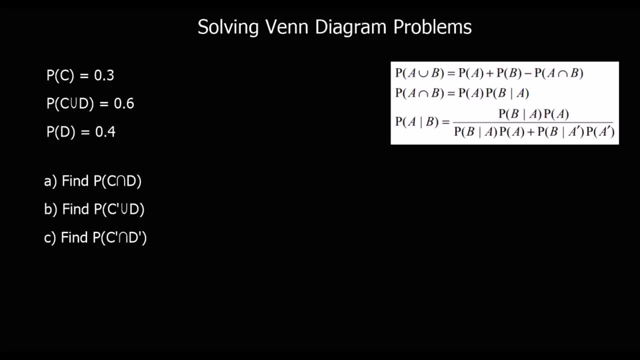 0.3.. Okay, here's another question. If you want to pause the video and go through this one, you can Otherwise Just keep watching, So I'm going to try and draw the Venn diagram first. again, I've got C and D this time. This time we've been given the union and not the, and so I'm 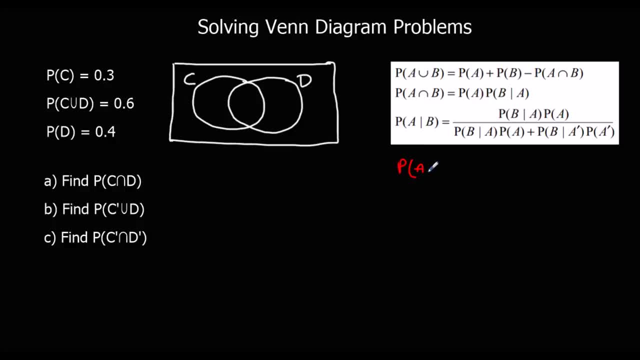 going to use the formula to get the probability of A and B, which would be probability of A plus probability of B Minus the union of A and B, So that will be 0.3 plus 0.4 minus 0.6, which will be 0.1.. 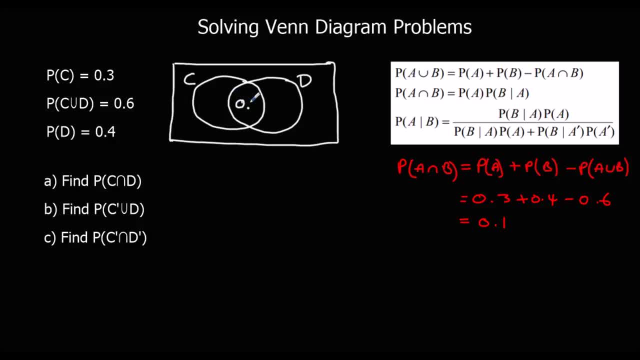 So the and section is 0.1.. And now we can just fill out the rest of the Venn diagram. So the probability. So the probability, The probability of C is 0.3.. We've been given, Well, we know the middle bit is 0.1, so we need another 0.2.. The probability of D is: 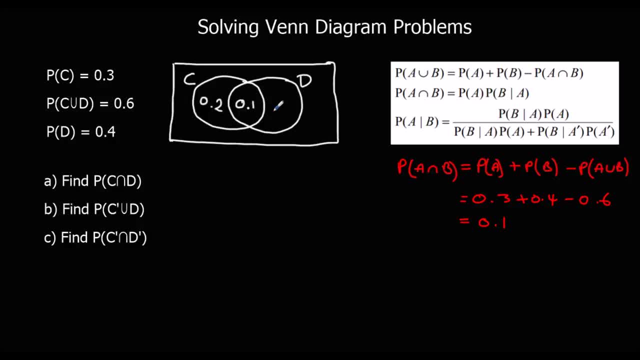 0.4.. We've got 0.1, so we need another 0.3.. And all of this adds up to 0.6, which means the outside must be 0.4.. Okay, the probability of C. 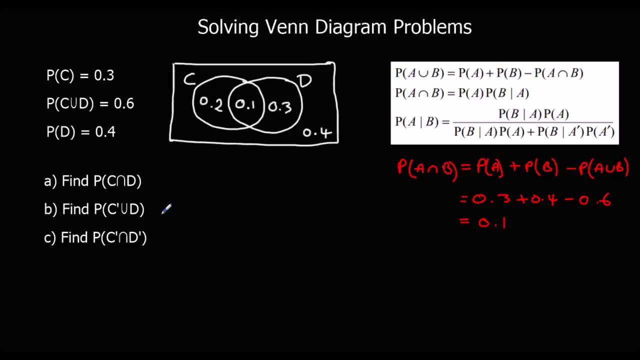 C and D. We've already worked that out. That was 0.1.. The probability of not C, the union of not C and D. So which bits are not C, These two are C, These two are not C And which bits are D. That's these two bits inside the D. 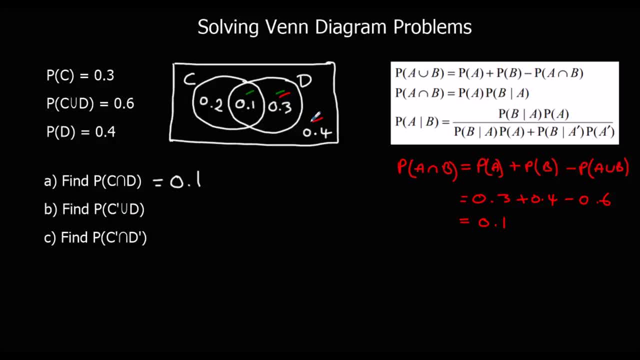 circle. So the union means everything I've marked with a line. So 0.1 plus 0.3 plus 0.4, that would be 0.8.. And if I get rid of these lines so I can draw some new ones, the probability of not. 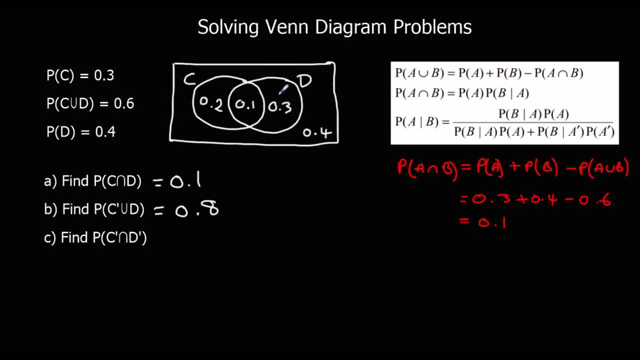 C and not D. So it's, and this time not C. That's those bits, Not D. These bits are D, So they're not D. Which bits? So it's, and So both of those things, The bit with both the lines. 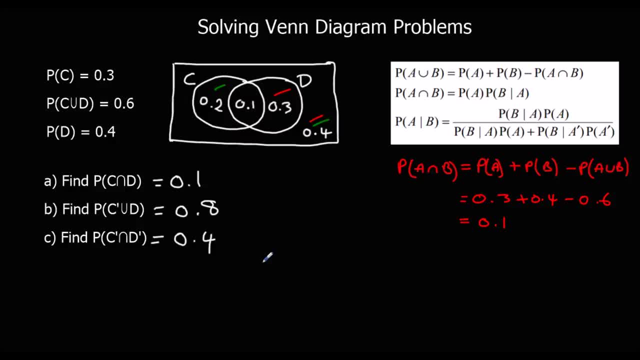 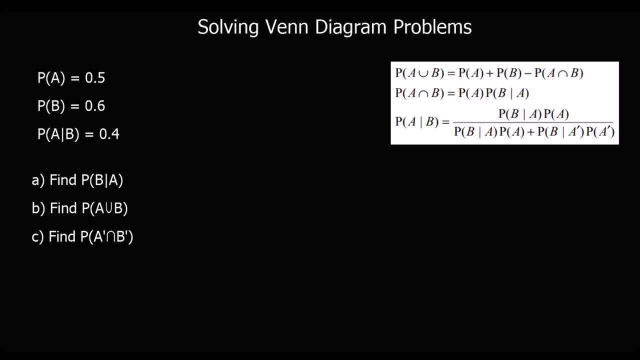 So that's 0.4.. Okay, this time we've got some given that information, So we're going to use that given that formula. So the probability of A given B is the probability of both of them together Divide by what's given. So the probability of B. 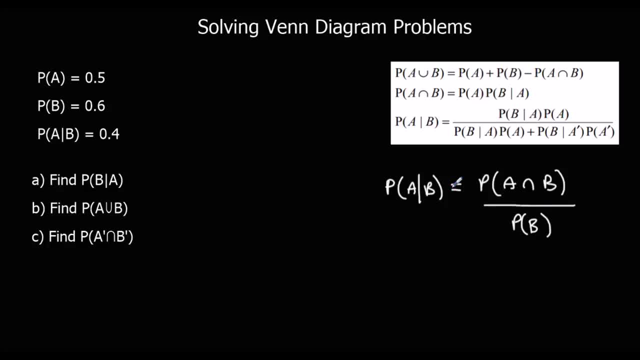 So we can find probability of A and B by timesing by probability of B. So the probability of A and B is probability of A given B times the probability of B. So in this case that's 0.4.. So that's 0.4.. 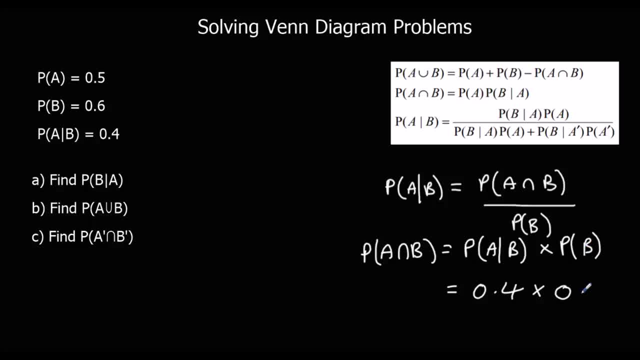 So that's 0.4.. Times 0.6.. Now, 4 times 6 is 24.. So 0.4 times 0.6. That's 0.24.. So we can draw our Venn diagram now. 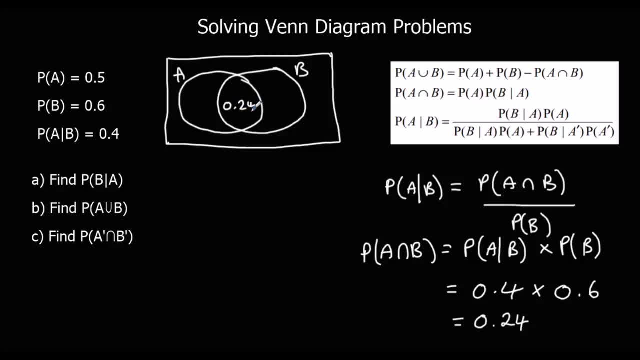 So the middle bit is 0.24.. The probability of A is 0.5.. We've already got 0.24.. So we need another 0.26.. The probability of B is 0.6.. We've already got 0.24.. 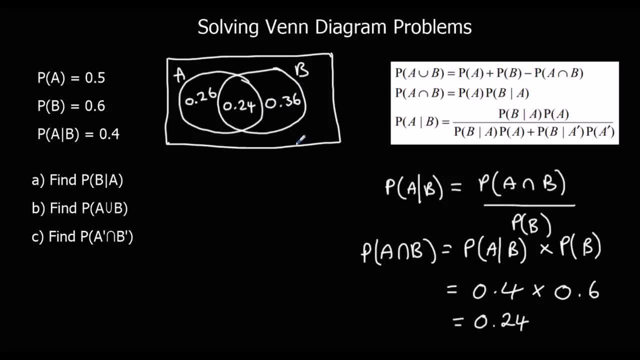 So we need another 0.36.. And the middle adds up too, So we've got 0.24 and 0.36.. Well, that's 0.6.. This circle is 0.6.. Plus 0.26.. 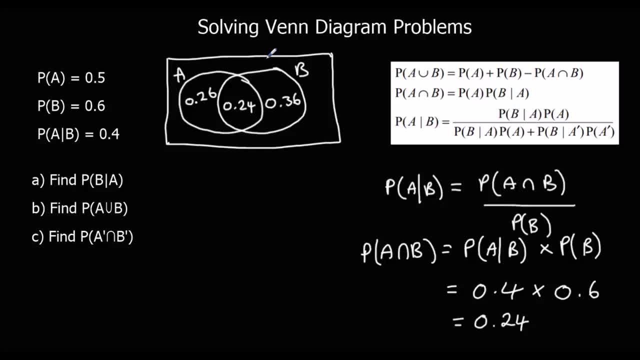 Is 0.86.. And that means we've got 0.14 left. 1 minus 0.86 is 0.14.. Okay, now we can answer the question. So the probability of B given A: Again, we're going to use this formula. 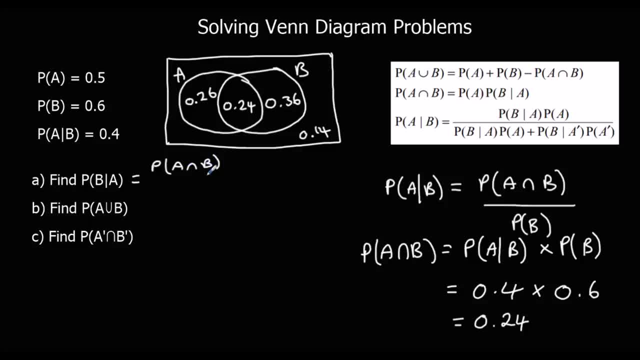 So that's the probability of both of them together Divided by what's given, So that's 0.24.. Divided by the probability of A, Which is 0.5.. And that will give us 0.48.. 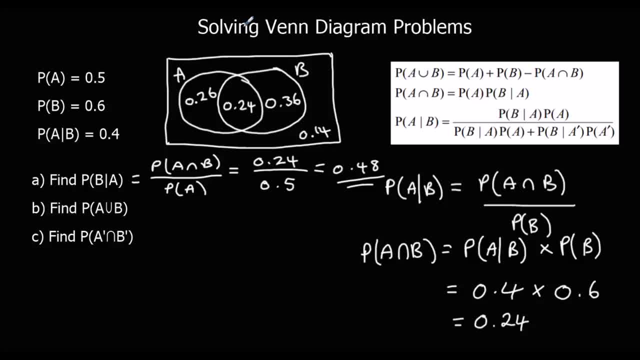 The probability of the union of A and B. So these two are A, These two are B, So the union is all three of these together, which is 0.6 plus 0.26, 0.86.. And I'll get rid of those lines. 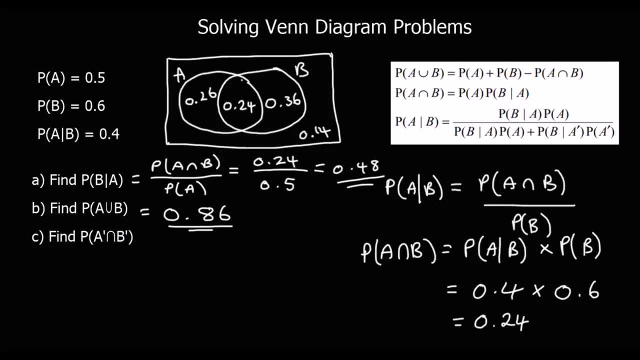 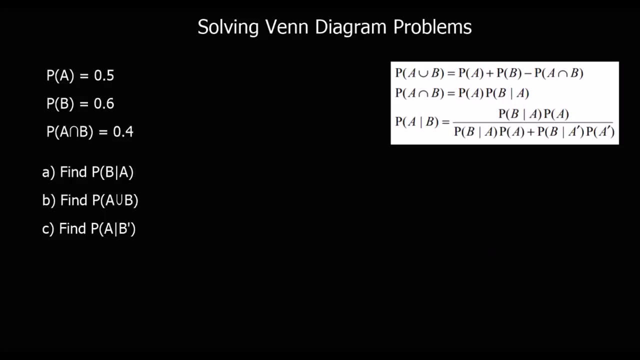 The probability of not A and not B. So these two bits are not A, These two bits are not B, Which is both of them 0.14.. Okay, one more question. If you can pause the video and give it a go, do that. 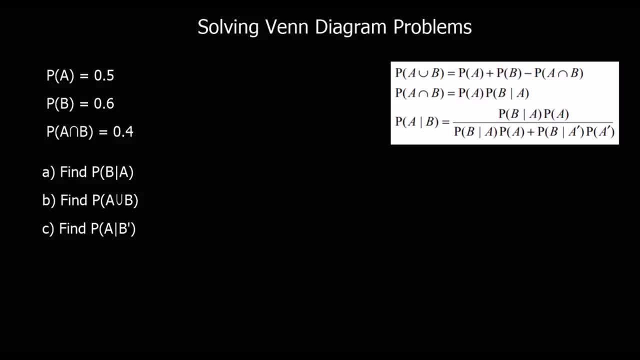 Otherwise keep watching. So we're going to draw our Venn diagram first. We've been given all the information we need, So we've got A and B. the middle bit. A is 0.4.. Probability of A is 0.5.. 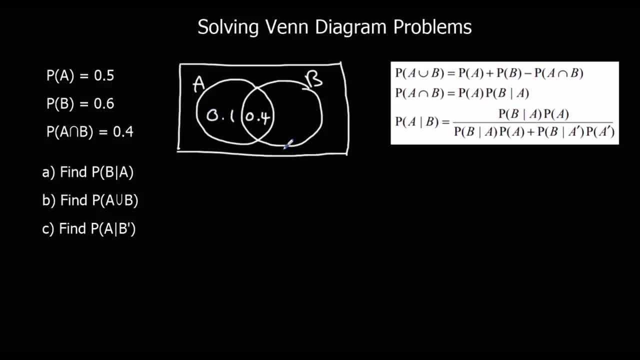 We've already got 0.4.. So 0.1 left. B is 0.6.. We've already got 0.4.. So 0.2 left And all of these add up to 0.7.. 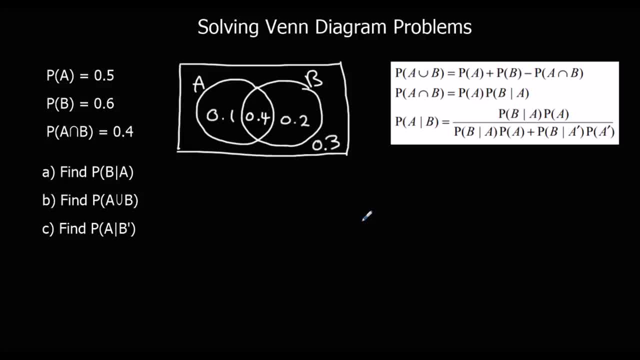 So we must have 0.3 on the outside. Okay, the questions Find the probability. The probability of B given A, That's the probability of both of them together Divided by what's given. So the probability of A and B is 0.4..